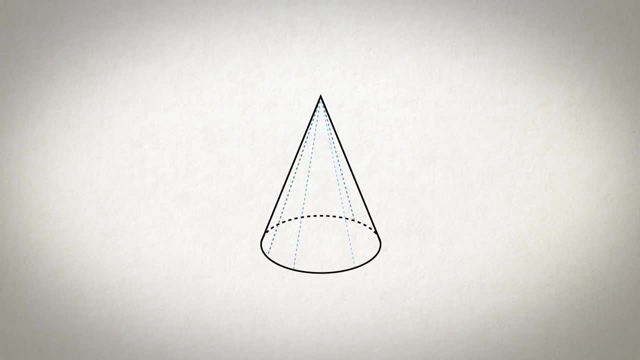 and on the geometric line. Let's now section it. Let's see We position the intersecting plane. Let's start with a plane that will section all the geratrixes. We shall obtain an ellipse If we straighten this plane, making it horizontal. 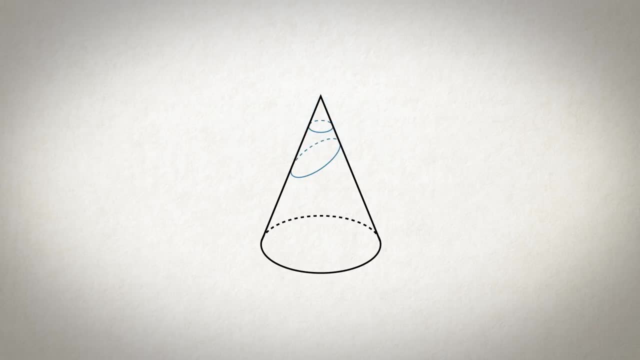 we get a circle, which is a particular case of the ellipse. Let's increase the incline. The intersection with a plane parallel to two geratrixes results in a hyperbole branch If we continue to tilt the plane until it becomes parallel with the g-line. 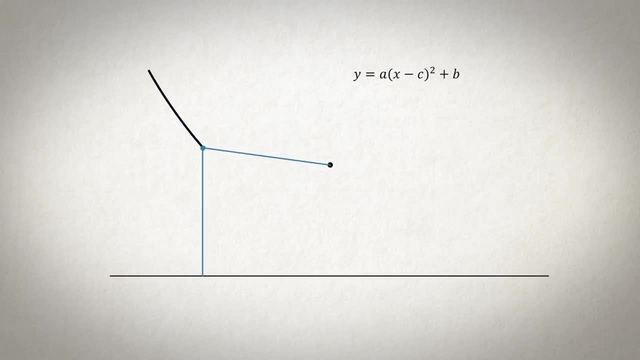 we then obtain a parabola. A parabola is the flat curve defined as the group of points that are equidistant from a point and a line. It's quite simple actually. We come across this line in our everyday lives, from shore to shore, on suspended bridges, in Portugal, the USA, in China. 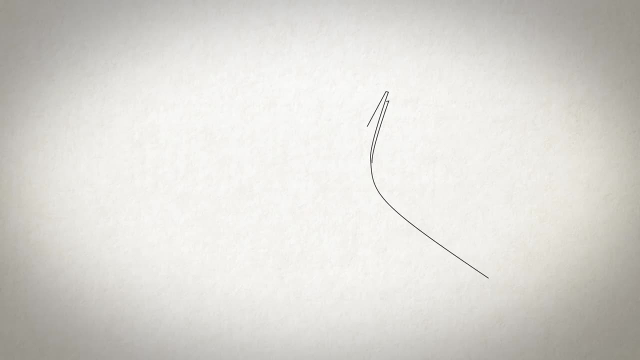 Let's now have a look at these three projects. The first, the Cathedral of Brasilia, by the architect Oscar Niemeyer. It was built between 1958 and 1970, and each of the 16 reinforced concrete pillars weighs in at 90 tons. Next, we have the Sagrada Familia School. 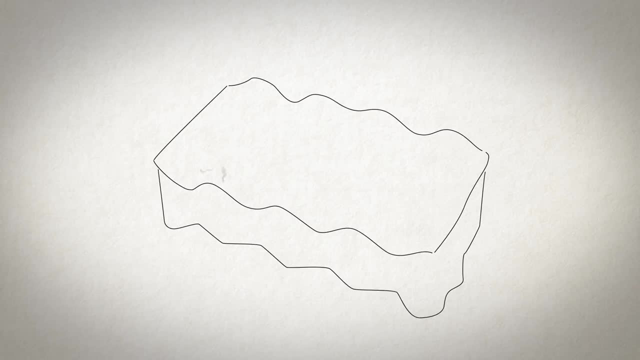 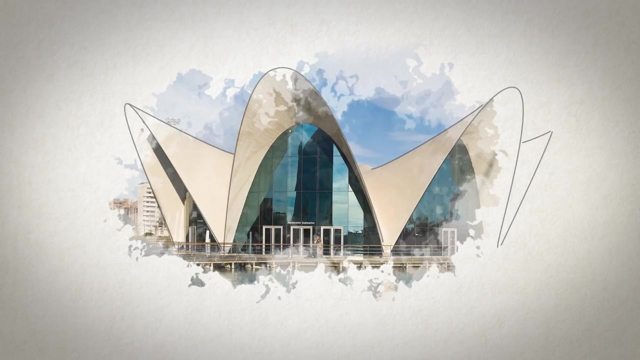 in Barcelona. The little building built in 1909, is a project of the last artistic stage of the Catalan Antoni Gaudi. And finally, the Oceanarium of Valencia, finished in 2002.. It was the last work of the architect, Félix Candela, who died at the age of 87 without seeing it completed. 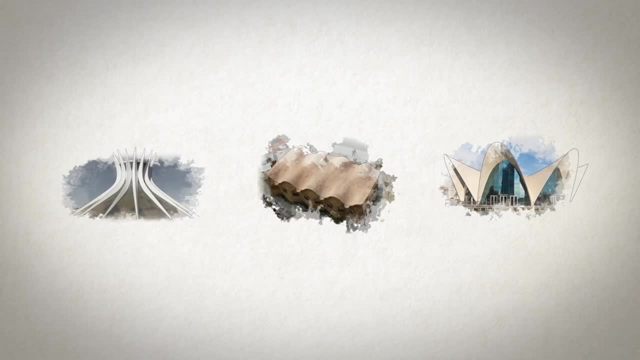 So what do these three projects have in common? The answer seems blatant, doesn't it? There are no straight lines, only curved meshes, right, Wrong, Or should we say partially wrong. Okay, let's open a parenthesis here. In 2002, the Spanish architect. 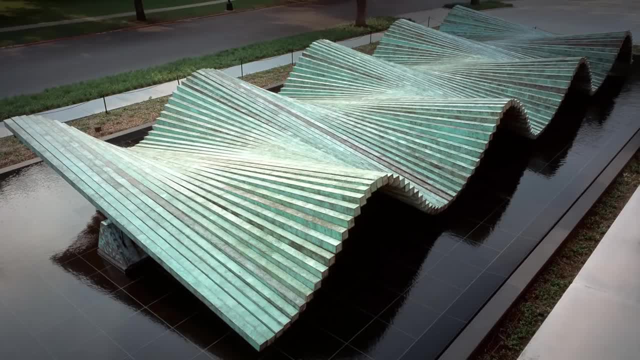 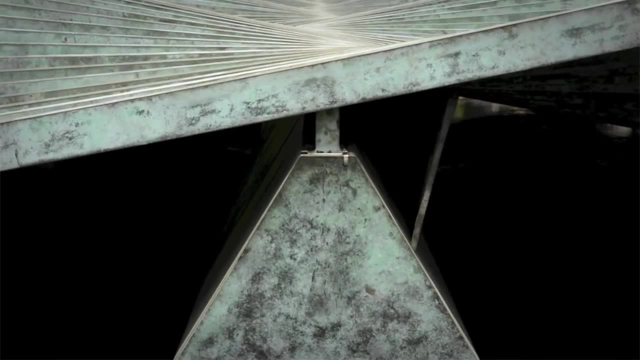 and engineer Santiago Calatrava inaugurates Wave, a sculpture ordered by the Medus Museum in Dallas. However, Calatrava didn't just create a common sculpture, but rather a kinetic piece whose movement creates a wave. The curved surface of the wave is suggested by the synchronized movement of 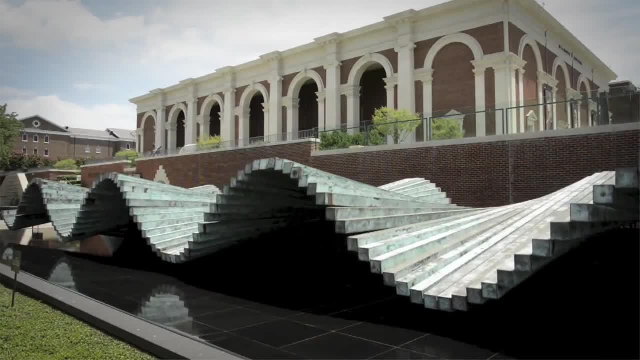 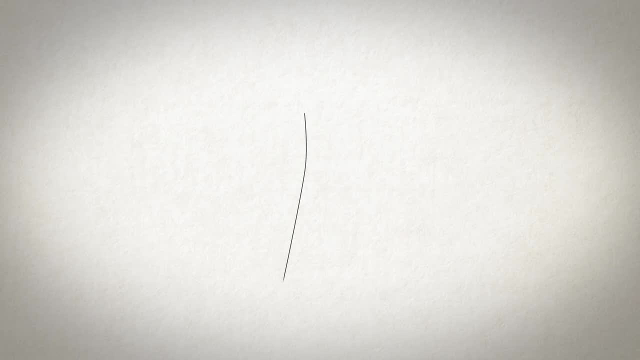 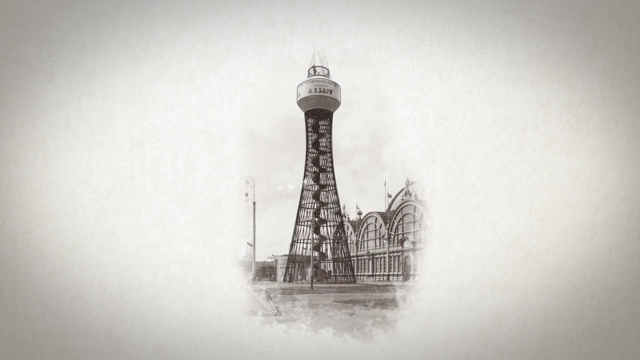 the wave in the shape of a wave. The wave has a diameter of 129 beams, mathematically positioned. How does this all work? Let's check with history. Vladimir Shukhov was born in 1853 to the then Russian Empire. In 1896, Shukhov built the first structure shaped like a leaf, hyperboloid, a 37-metre. 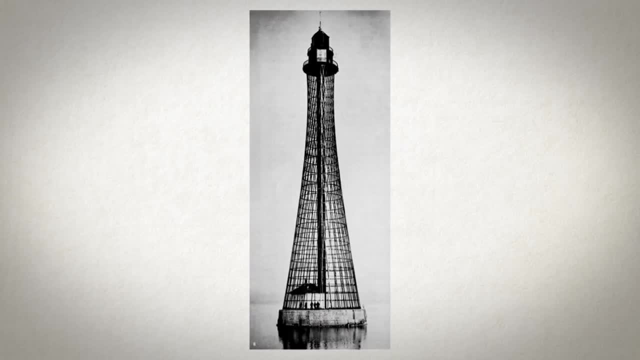 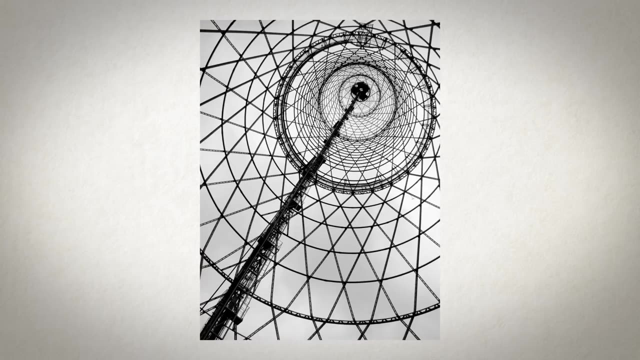 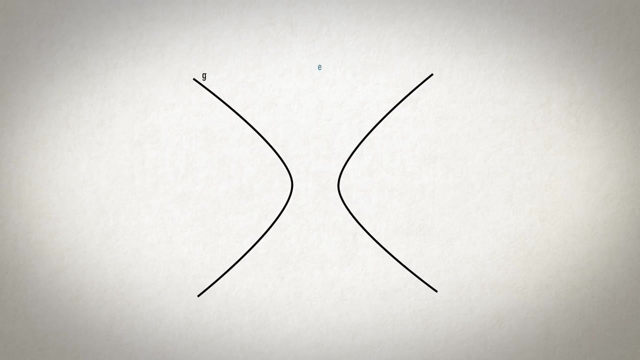 light steel tower sustaining a water reservoir on the top. Shukhov is considered the inventor of a family of structural shapes, the one-sheet hyperboloids of revolution. So what exactly are hyperboloids of revolution? We'll need a hyperbole which will function as a geratrix, We'll need an axis, and now the hyperbole. 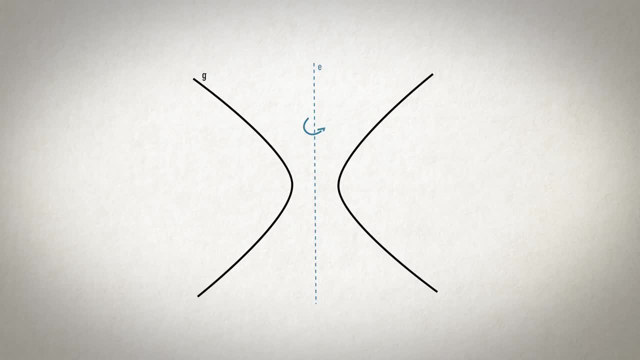 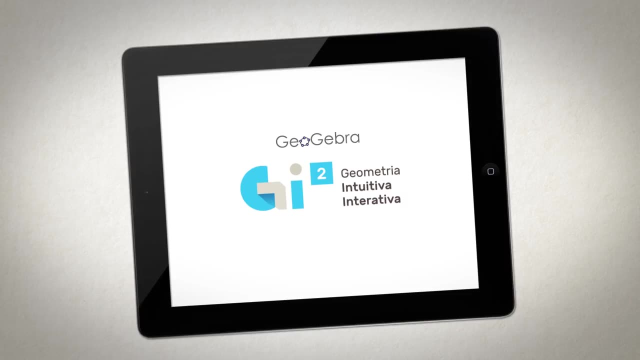 will execute a revolution around the e-axis. Let's make use of the GeoGebra, through the GI Alquadrado site, to help us with the tridimensional simulation. The full revolution of the curve around the axis has generated what we call the one-sheet hyperboloid of revolution. 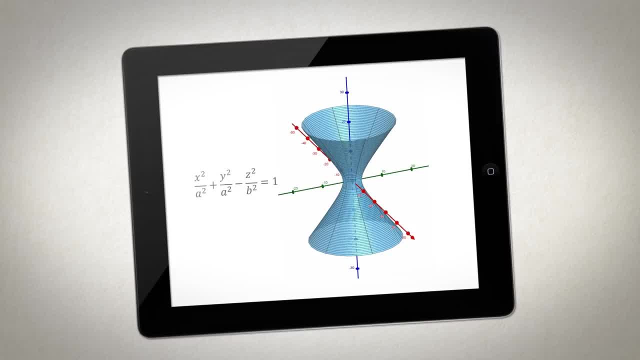 And what about that initial question of ours? Is it just a curved surface or does it contain straight lines? For each of the points of the hyperboloid, two distinct lines run through and are contained in the surface. So it's confirmed. The one-sheet hyperboloid of revolution combines the curve-shaped with the twice-ruled structure. 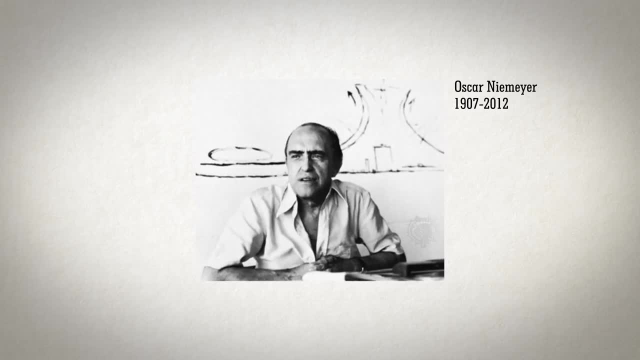 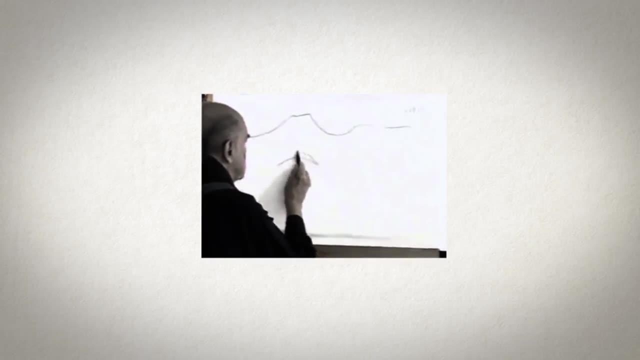 It is now time to go back and contemplate Oscar Niemeyer's curves. Niemeyer said that what attracted him was the constraint-free and sensual curve, the curve he found in Brazil, in a sinuous state of the ocean and in the body of the favorite woman In Niemeyer. purity of architecture comes. 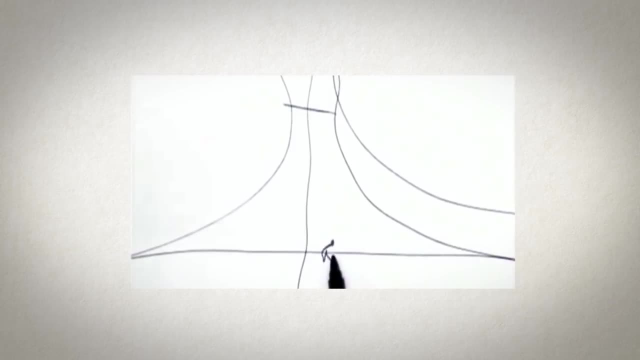 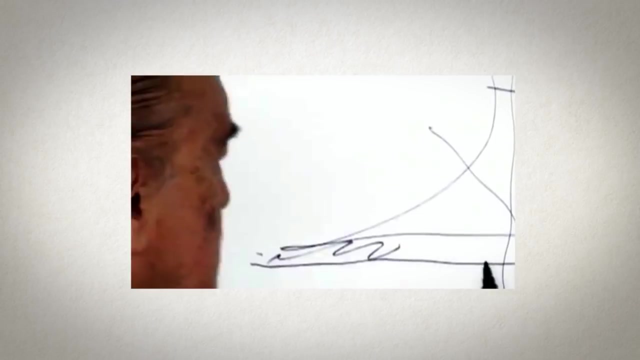 down to this simple gesture, a poem, and the curve In the Cathedral of Brasilia. in accordance with the concept of architecture, the shape and arrangement of the pillars represent two hands lifting towards heaven. Though, while Niemeyer drew the ideal shapes which would transport the 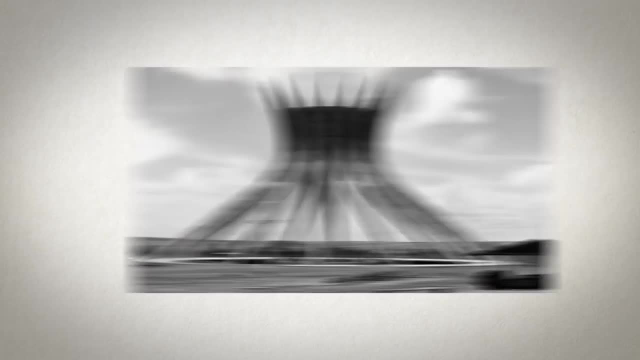 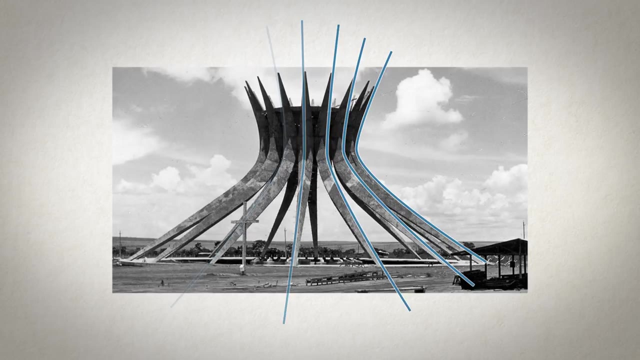 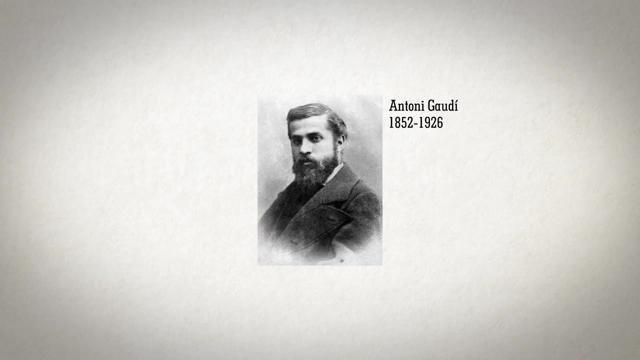 Catholic to infinity. Joaquim Cardoso, the engineer specialized in structural calculation, which made the Brasilia ideas possible, pondered over the best hyperboloid which best solved the problem. Andoni Gaudí is one of the most famous architects in the history of architecture. 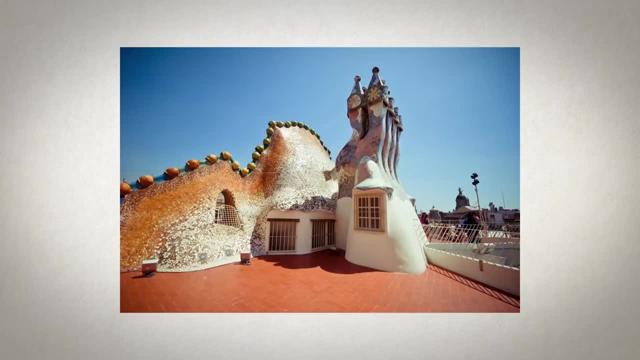 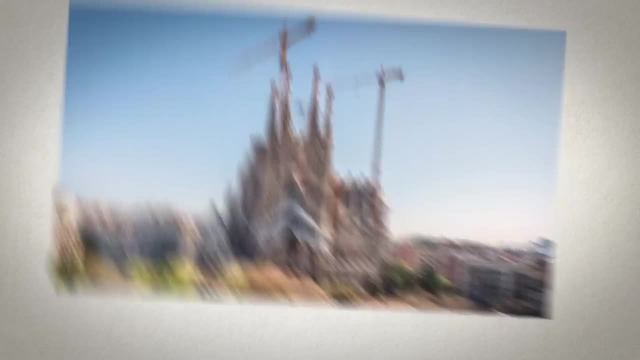 His work primed in the use of organic and naturalistic, which in itself set it aside from the then-architectural tendencies. His first work of art, the Sagrada Familia, is still today, 135 years after its start, in progress. Gaudí had a passion and a knowledge. 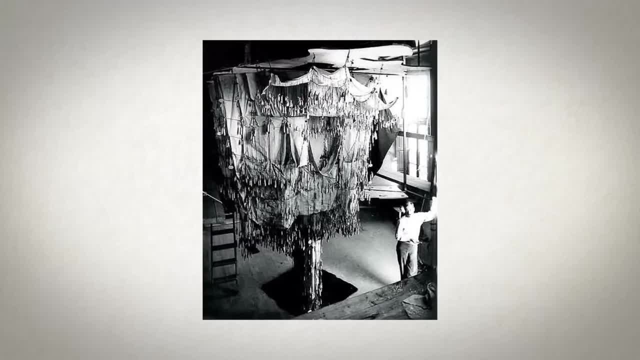 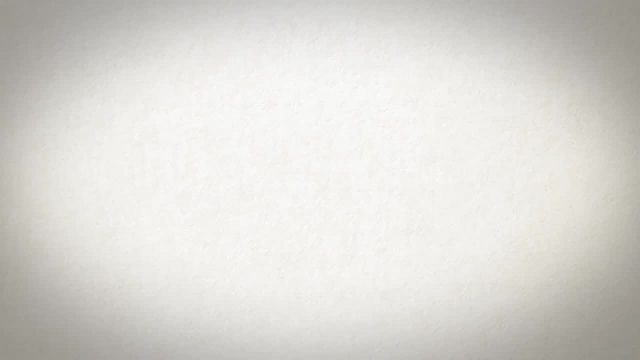 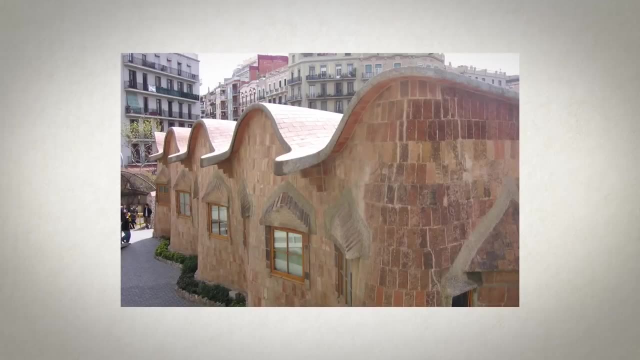 for mathematics and geometry, which allowed him to develop new structural systems without recurring to calculations. He tested his stress models in scaled-down models, which he then applied in his work. Gaudí was the first architect to use kenoids in his work. Presently, and in his honor, they are called Gaudí-ruled surfaces. 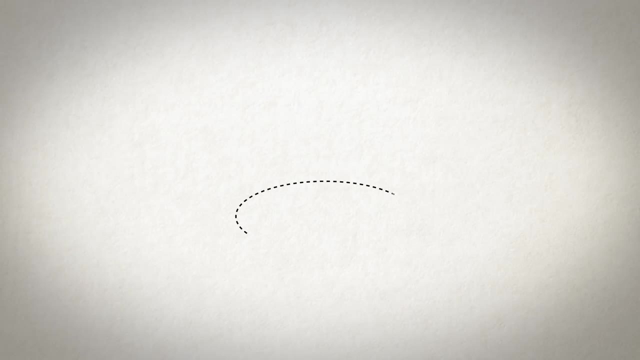 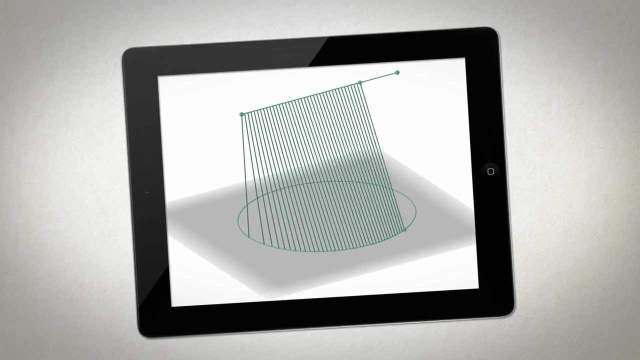 Let's now explain how a kenoid is geometrically generated. We shall use as the directrix a circumference D, We'll use a line, segment E, as an axis And, finally, the line G will be the geratrix and shall lean on the axis and the directrix, moving through them and generating the kenoid. 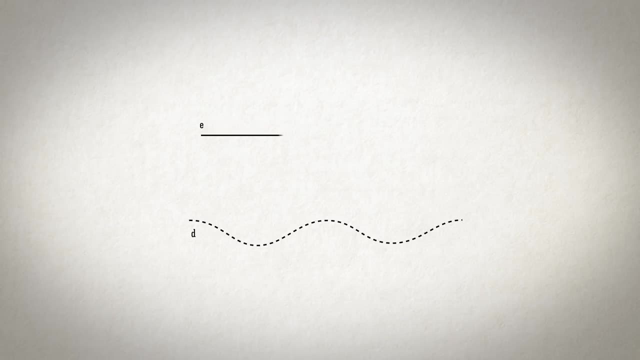 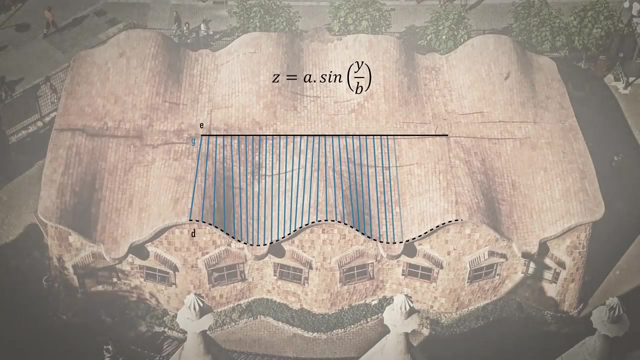 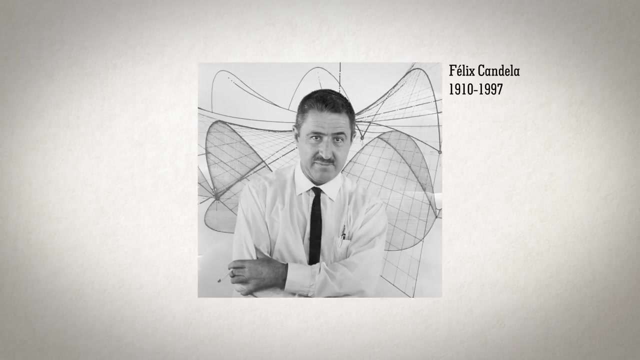 Let's make a second experiment. Instead of a circumference, let's use a sinezoidal directrix to generate a sinezoidal kenoid, the kenoid that Gaudí applied in the wall and roof geometry of the Sagrada Familia school. Félix Candela was born in Spain, but at 26 he leaves for Mexico. 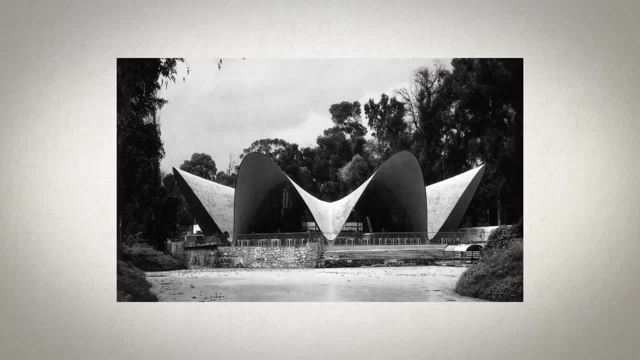 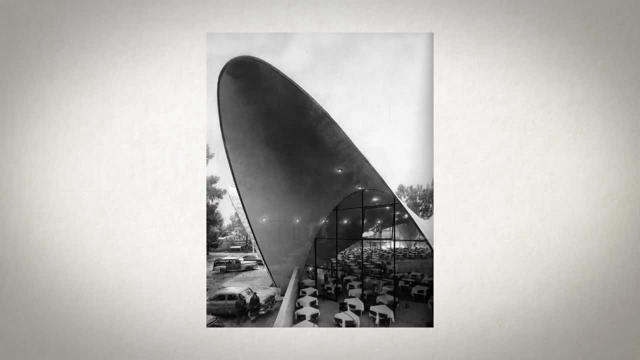 where he takes up double citizenship. Candela had a special talent for geometry and an oath with the surface called hyperbolic paraboloids, with which he frequently resolved his architecture. Candela sustained that the geometry of this surface generated the necessary rigidity to enable 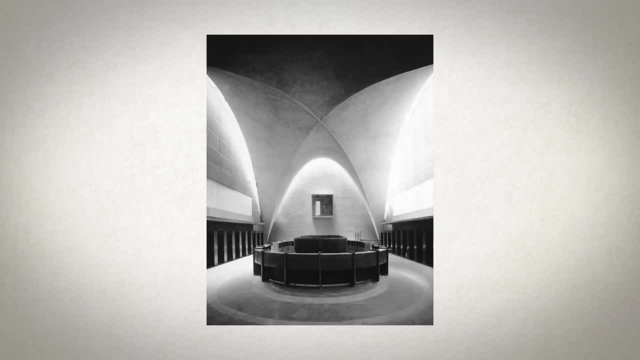 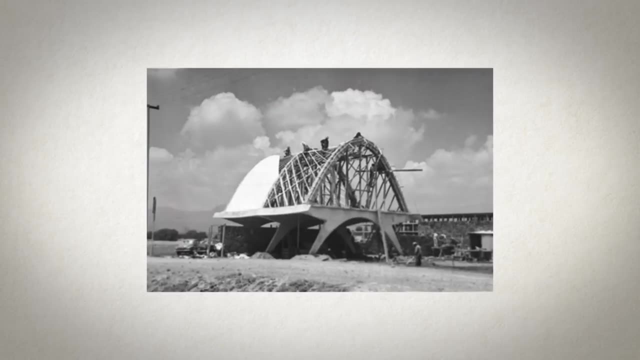 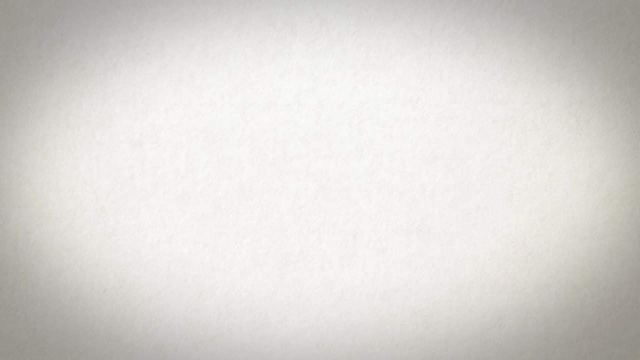 the construction of blades with minimum thickness, the so-called cascarones, Built in 1951, the Cosmic Race Pavilion, a small laboratory in Mexico City, was his first work employing this surface. This membrane of concrete was only two centimeters thick. So what is a hyperbolic? 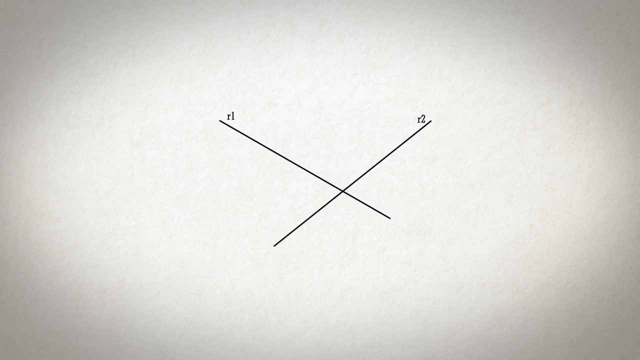 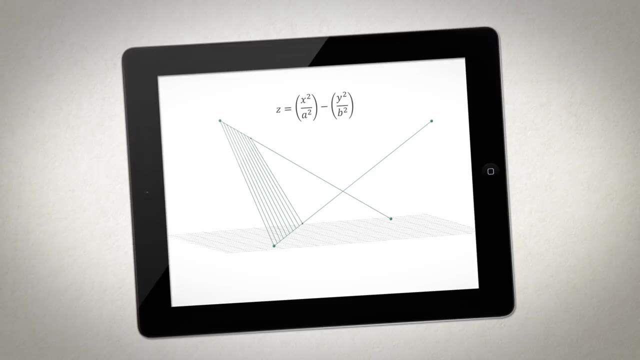 paraboloid. Well, we'll need two non-complainer lines, R1 and R2.. Let's run a third line, G, through the other two. Now all we have to do is move the G line at constant speed through the R1. 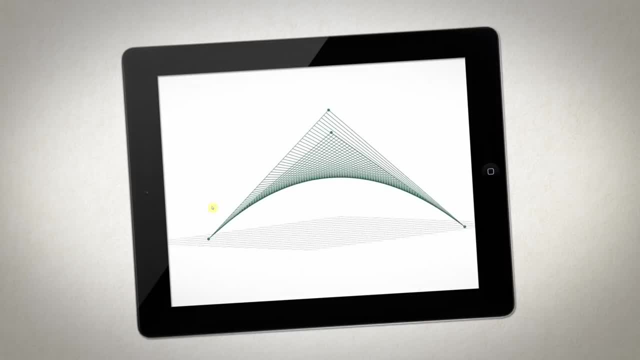 and R2 lines, obtaining the twice ruled surface. The hyperbolic paraboloid name is due to the fact that it has both hyperboles and parabolas as sections. Let's see: By sectioning this surface with a horizontal plane, we can now draw a line that is equal to the horizontal plane of the surface.